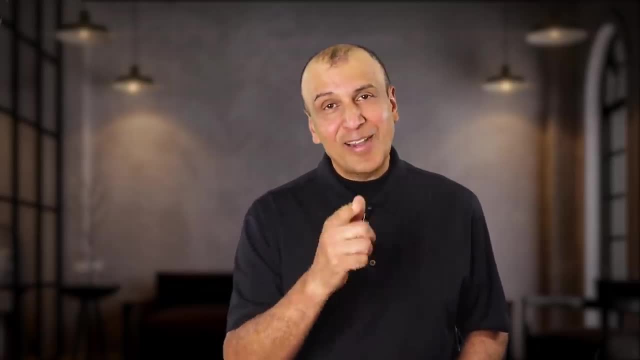 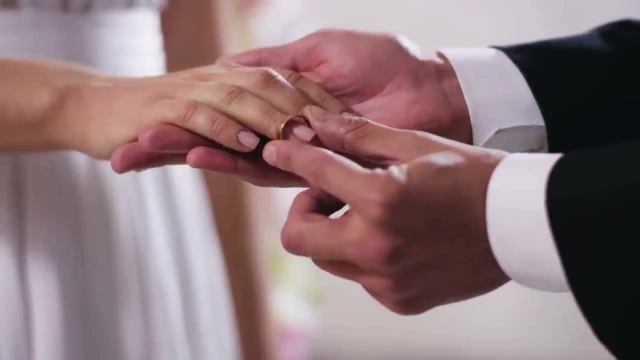 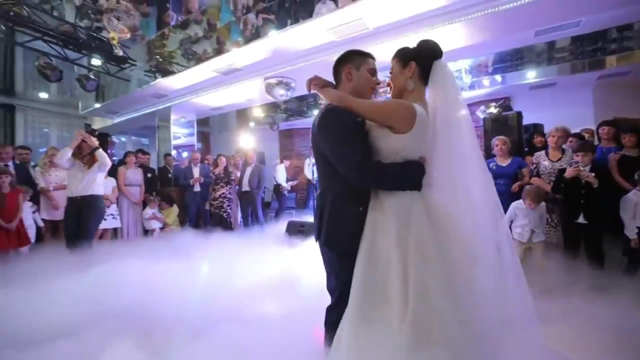 it a little bit better, And that's coming up right now: Entanglement sounds sort of like entanglement, but it's more like entangled pairs of people. If Alice and Bob get married, they literally become entangled by tying the knot. Suppose that then Bob tragically dies, Alice goes. 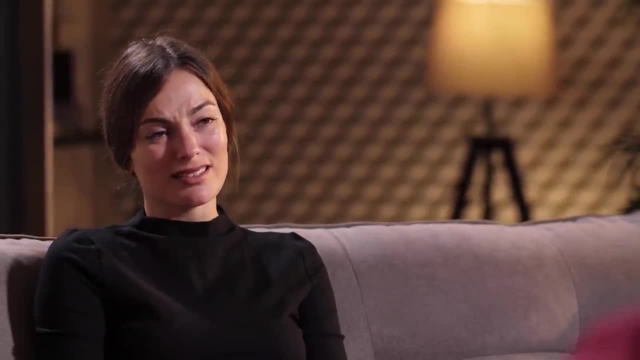 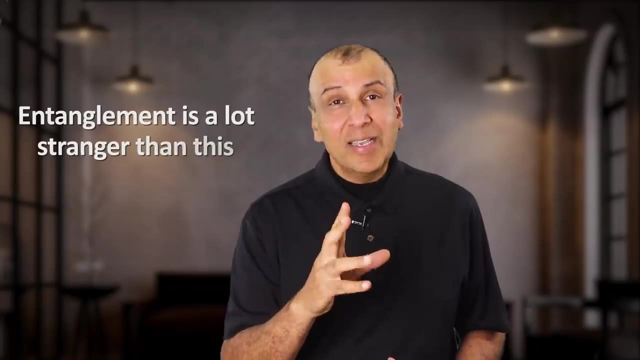 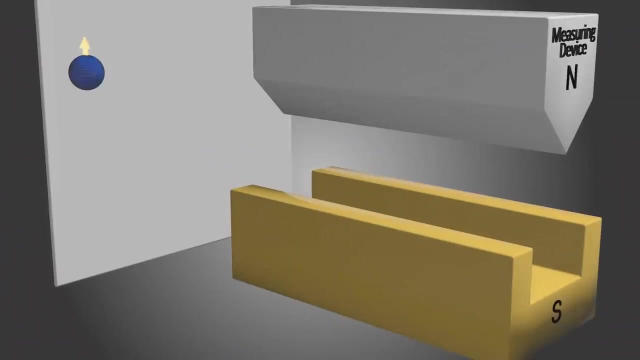 from being a wife to a widow. What happens to Bob changes Alice's status too. But what entanglement means for quantum particles is a lot stranger than this, And here's why. Imagine the particles are electrons, which have a quantum property called spin that makes them. 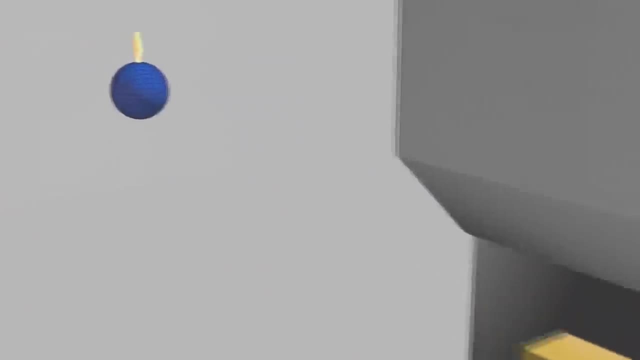 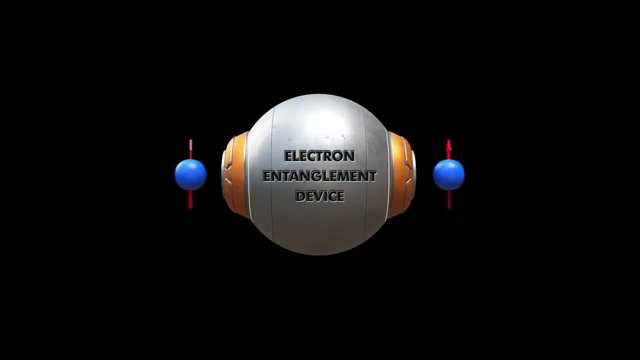 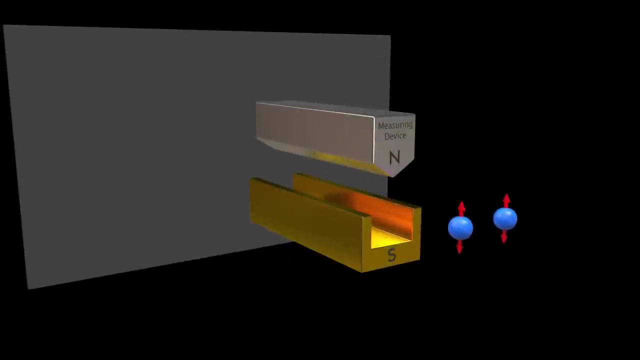 act like little magnets. If we measure this spin for an electron, we'll always find it pointing in just one direction or the opposite- up or down. say Now we can imagine entangling two electrons so that their spins are always pointing in opposite directions. If electron 1 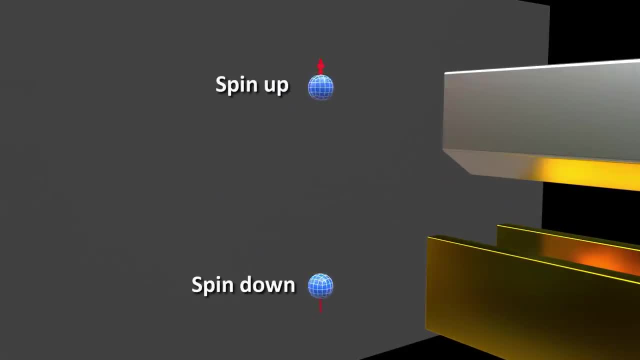 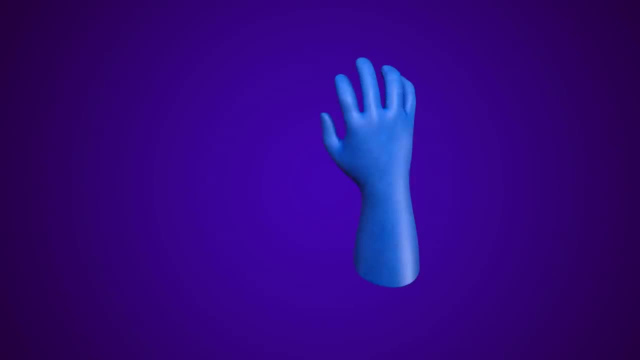 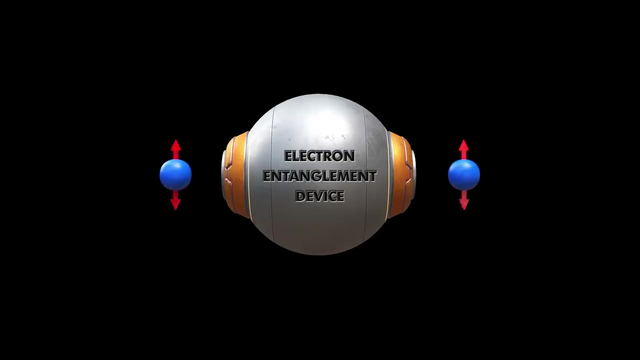 has a spin up, electron 2 must have a spin down, and vice versa. The two spins are said to be correlated. They are like a pair of gloves: If one is right handed, the other must be left handed. So now, let's say we entangle the two electrons in this way. 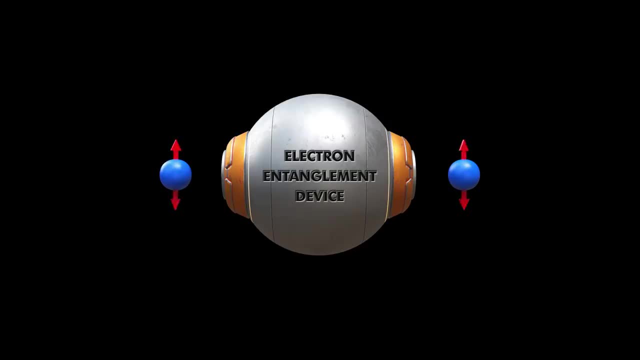 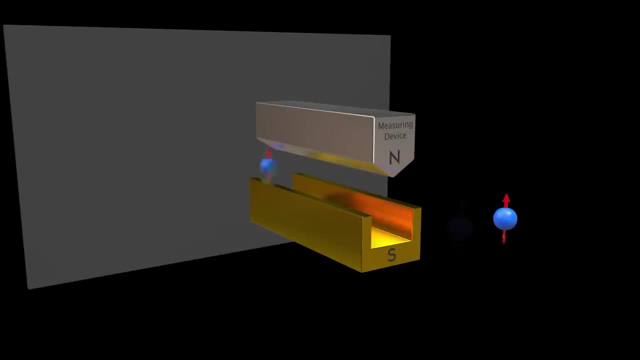 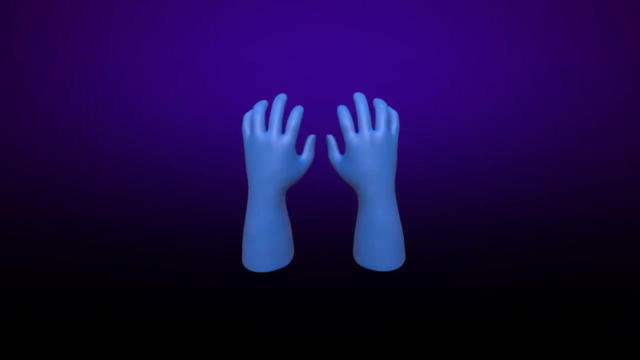 and fire them in opposite directions. We don't know which of the pair is up and which one is down until we make a measurement. If we find that electron 1 is spin up, we know the spin of electron 2 must be down. This is not remarkable, because we could do the 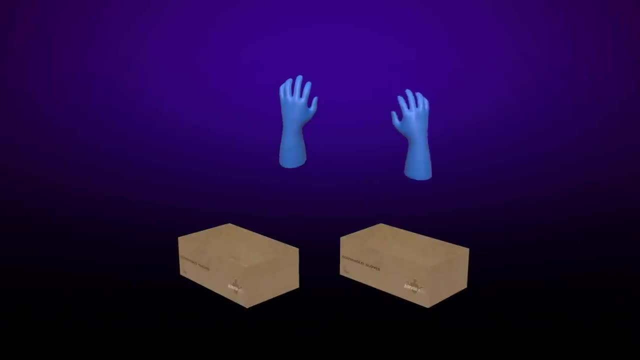 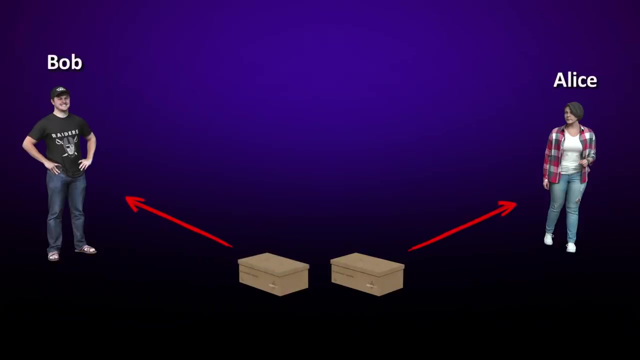 same thing with the gloves. We could put one in a package and send it to Alice and the other to Bob. The moment Alice opens her package and finds the right hand glove, she knows Bob must have the left hand glove. The handedness of the gloves, like the spins. 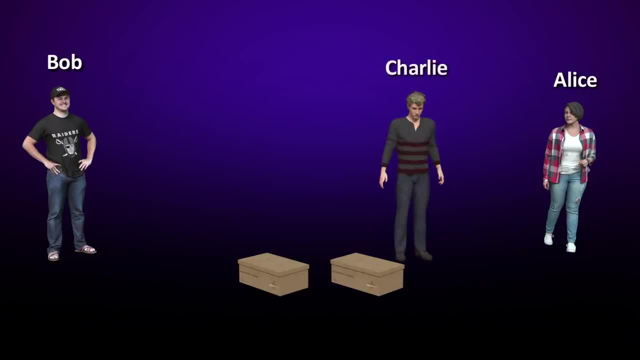 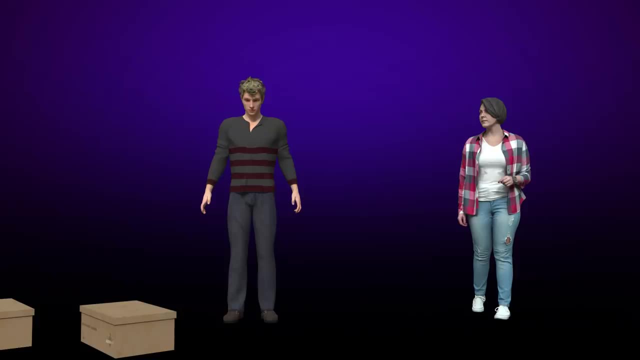 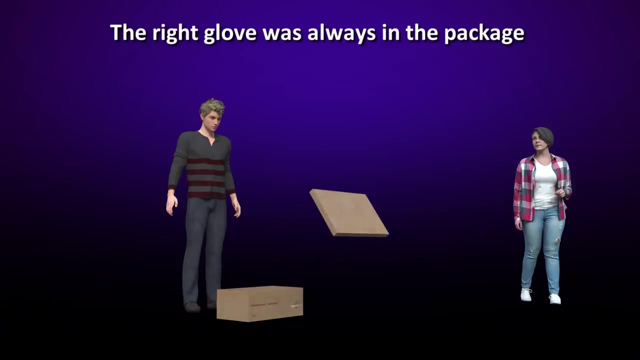 of the electrons is correlated, But there's a crucial difference in this analogy. The handedness of the gloves in the package was the same from the start. It never changed. It was always the right hand glove that got sent to Alice. If someone had intercepted the parcel before Alice got it, that person got the gloves. 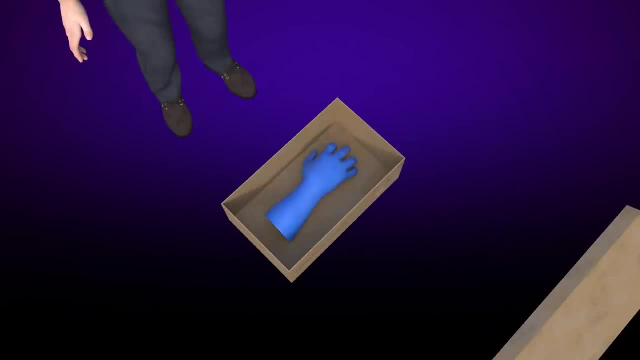 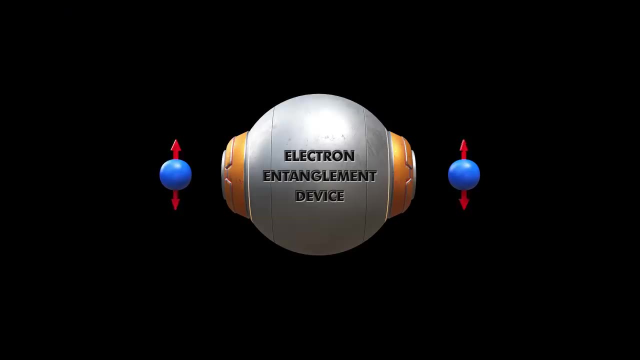 person would have seen that it was the right-handed glove With entangled particles. that's not the case. Remember, all we did at the outset was ensure that the entanglement made them correlated so that their spins point in opposite directions. We didn't specify whether the 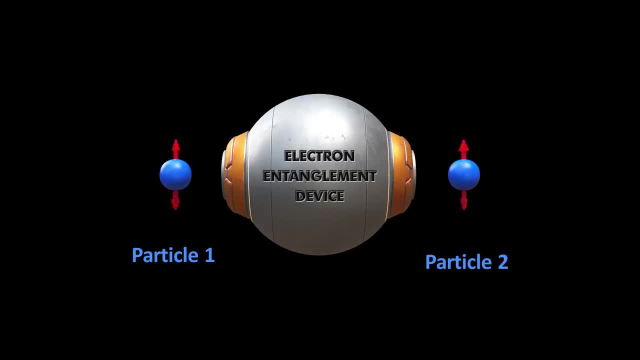 spin-up electron is number 1 or number 2.. You might think: well, ok, it's obviously one or the other. It's just that we didn't know which was which until we measured one of them. Well, that's not quite the case. Say, we set up an electron so that it could. 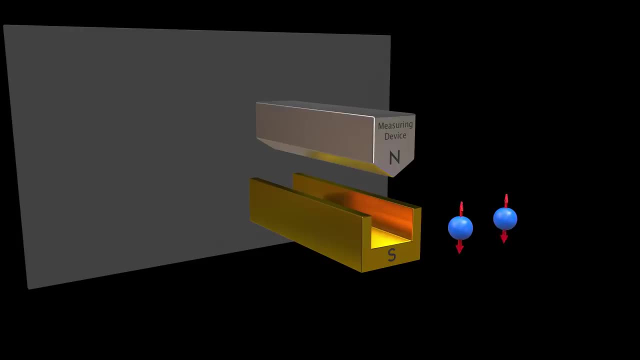 have either spin-up or spin-down when we measure it. That's called a superposition. Then the electron's spin orientation simply isn't described until the measurement is made. It's not just that we don't know it yet. There is no definite answer one way or the other. 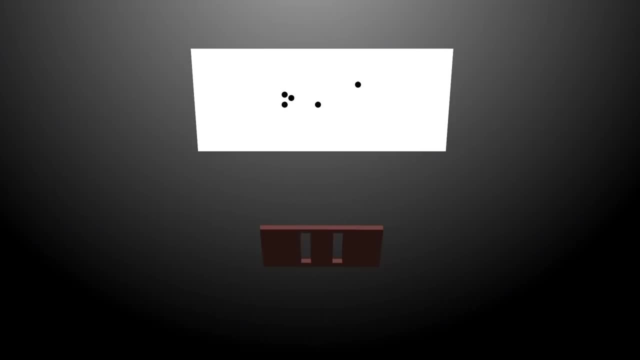 How do we know that superposition is real and not just an illusion? due to our ignorance? Well, first of all, we don't know. How do we know that superposition is real and not just an illusion? due to our ignorance? How do we know that superposition is real and not just an illusion? due to our ignorance? 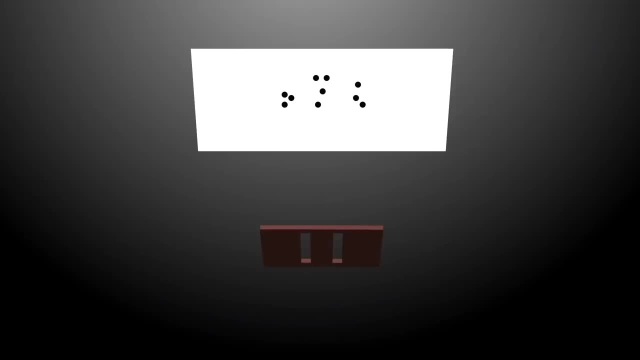 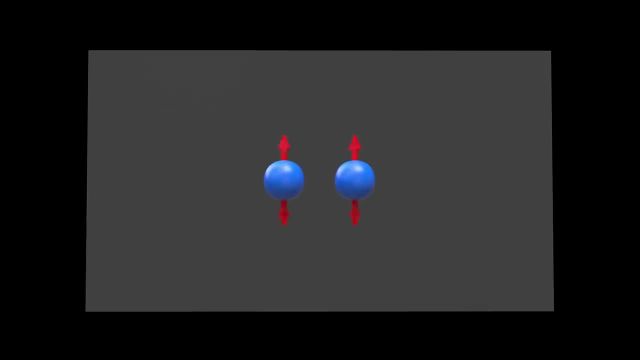 One experimental clue comes from a double-slit experiment. This experiment shows that a particle is indeed spread out like a wave that can be in many locations prior to measurement, But after measurement the particle becomes distinct and localized. This phenomenon is weird enough just for a single particle, But with entangled particles it's even weirder. 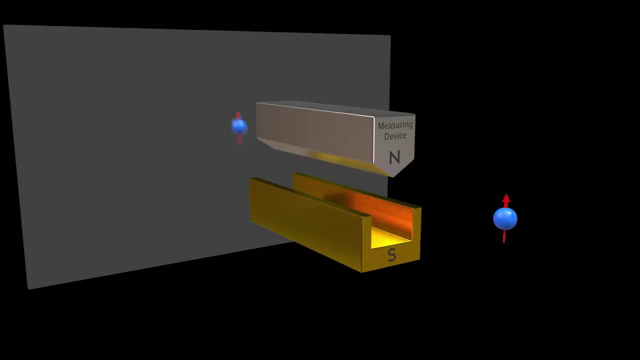 Because it then seems that a measurement on one particle determines the outcome not just for that particle but for the other particle- And that's what we call a superposition- But for both of them. When we only measured electron 1, the measurement not only forced, 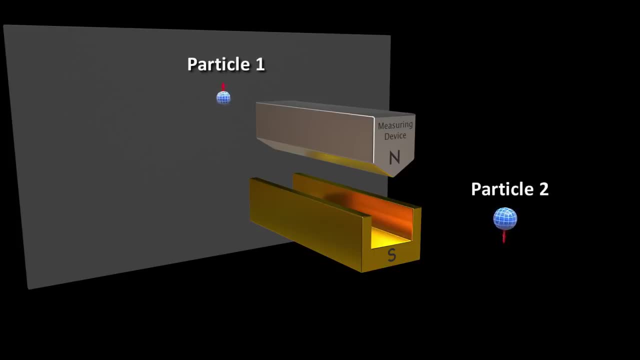 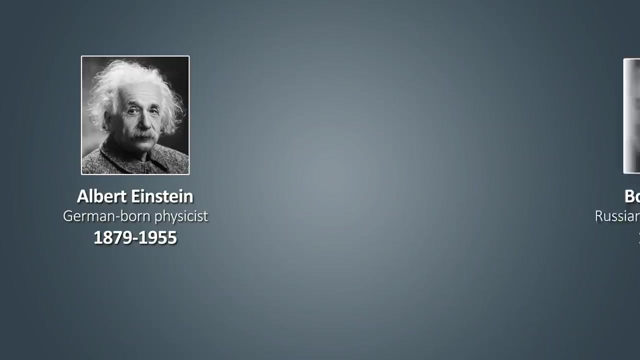 the universe to choose between spin up and spin down. for that particle, it forced the opposite choice for electron 2 because of their correlation. Albert Einstein thought up an experiment like this in 1935 in collaboration with two younger scientists, Boris Podolsky and Nathan Rosen. They are referred to as EPR for short, but 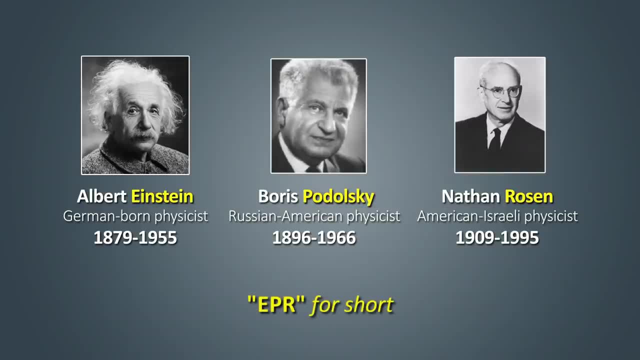 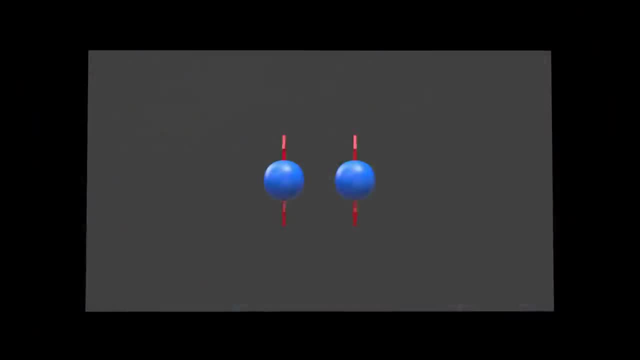 by combining the first letters of their last names. They didn't do this to show how weird quantum mechanics is. They did it to show that quantum mechanics could be incomplete. In this experiment, it looks as though by making a measurement on particle 1, we're. 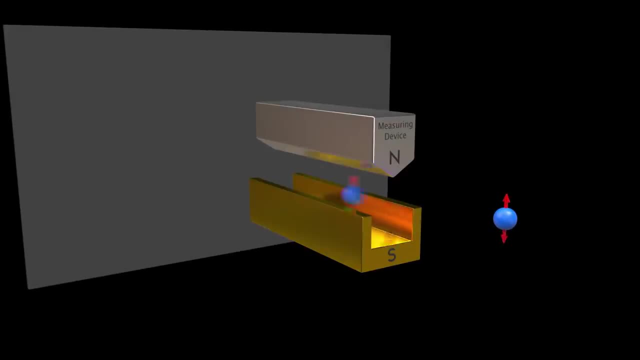 triggering some effect that influences the spin of particle 2. And according to quantum mechanics, this happens instantaneously. It takes no time for the effect to be felt by the other particle. But that's impossible Because I'm not sure if quantum mechanics 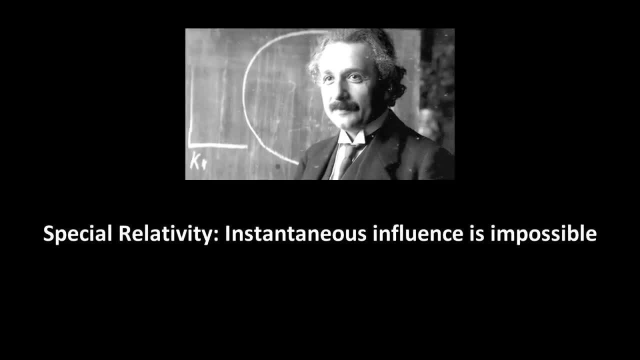 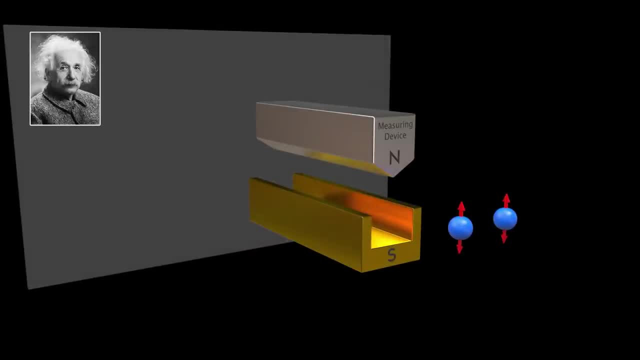 can do that? Einstein's theory of special relativity, devised 20 years earlier, said that no influence can be transmitted faster than the speed of light. It was as if, as Einstein said, there was some impossible spooky action at a distance that passed instantly between particle 1 and 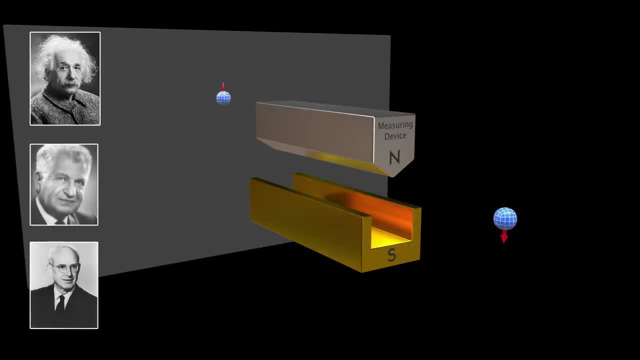 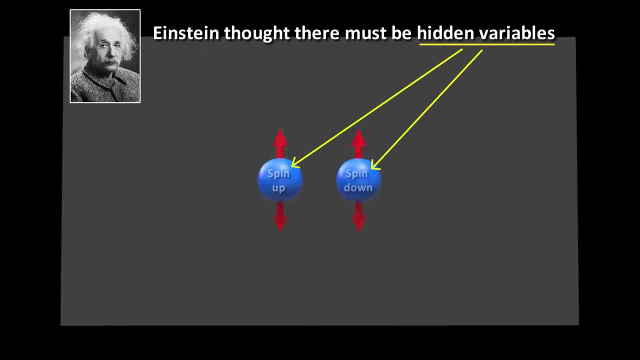 them, And they did, But they didn't. They figured that there must be a way to measure them, Something- what Einstein called hidden variables- that fixes the orientations of the spins all along, And that we couldn't actually measure these variables to find out the orientations. 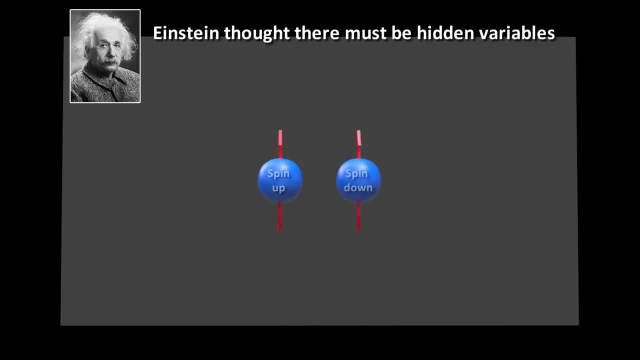 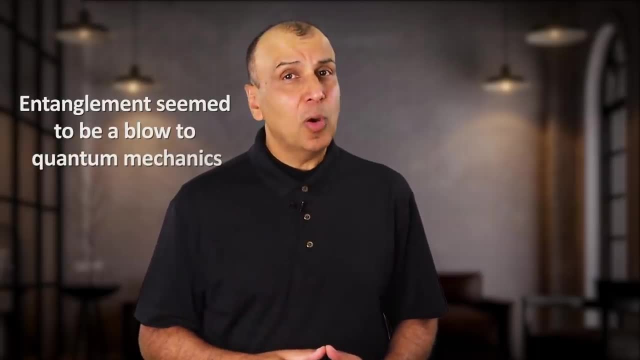 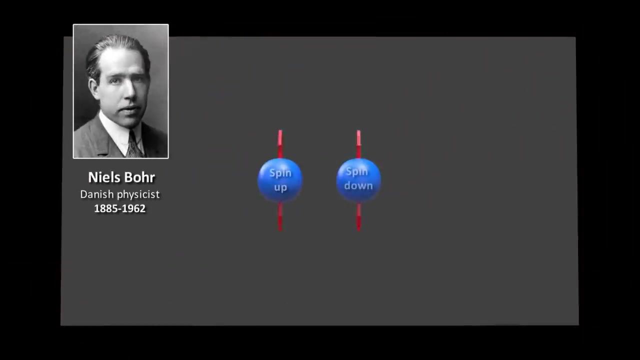 of the spins. That's why they are hidden. But they must exist, according to EPR. So the phenomenon that they had discovered, which became known as entanglement, seemed to blow a hole in the logic of quantum mechanics. But others, like Danish physicist Niels Bohr, said that Einstein was just wrong. Bohr said: 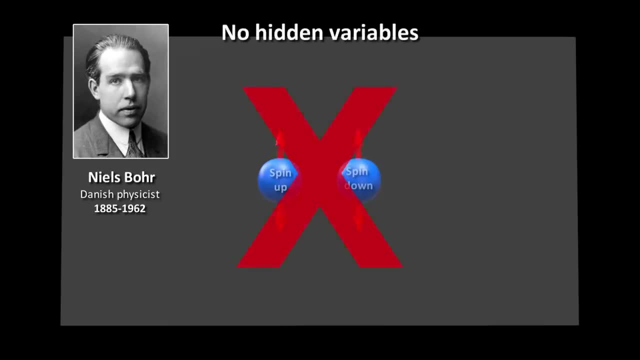 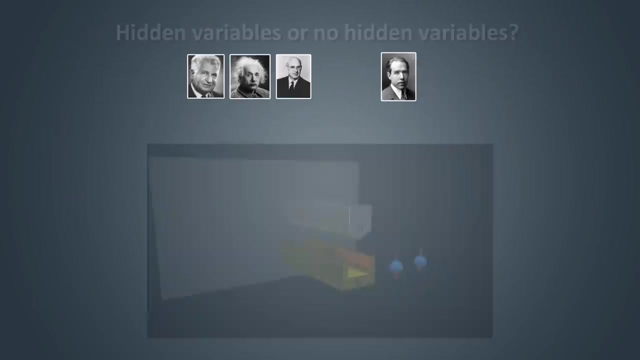 Bohr said there were no hidden variables, and the fact that entanglements seemed to create these weird correlations between particles was just something we had to accept as reality. There was no obvious way to tell who was right. Scientists remained divided. It was no good just doing the 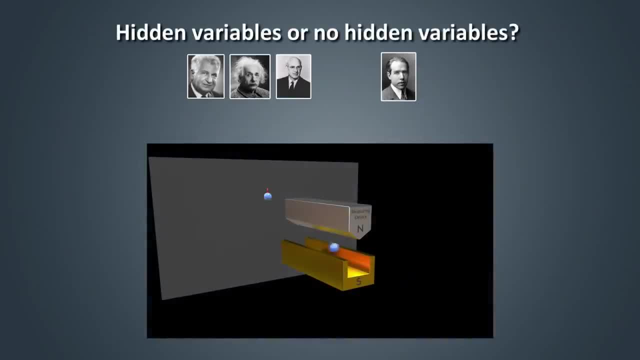 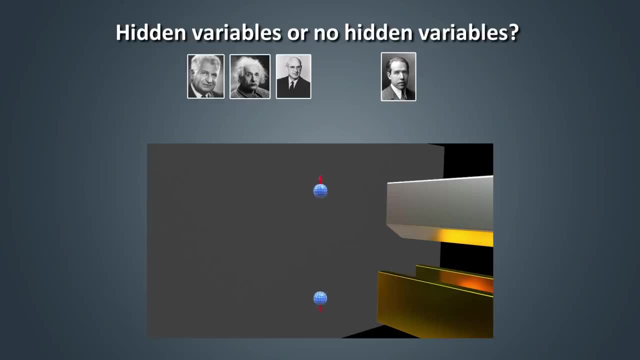 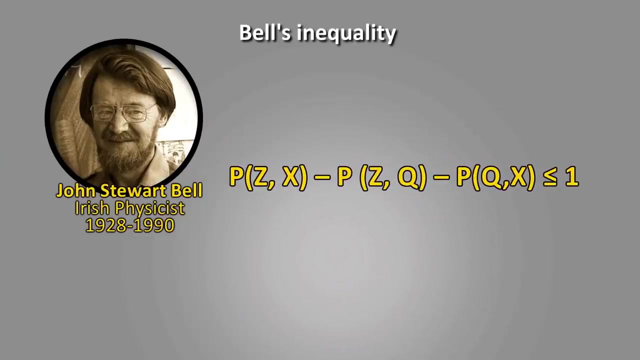 experiment that EPR had proposed, because simply measuring the spins wouldn't tell you if those spins had been fixed all along, as EPR thought, or whether they snapped into place after measurement, as Bohr thought. It wasn't until almost 30 years later, in 1964, that Irish physicist John Bell 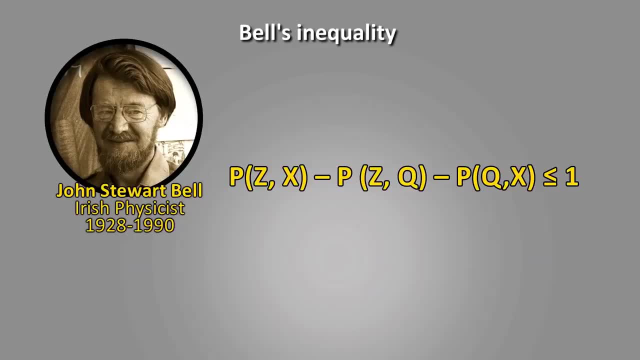 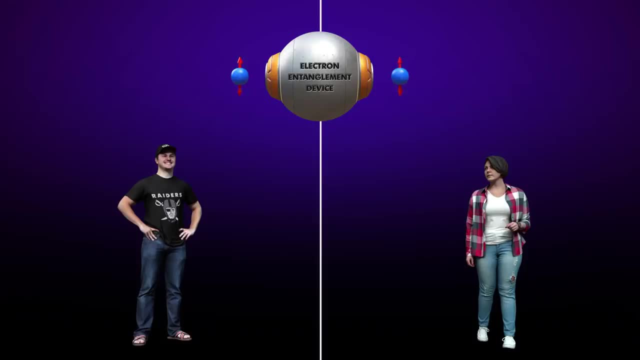 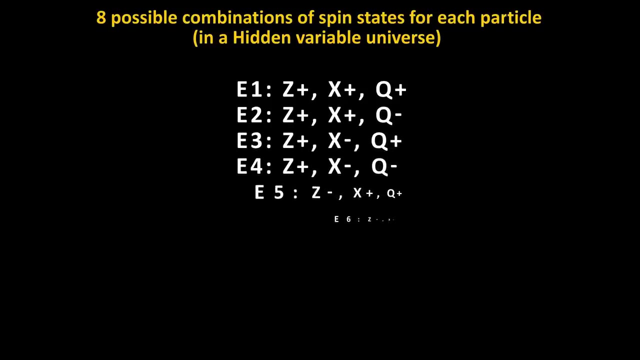 figured out how to set up a clever experiment to determine who was right. It involved running the experiment again and again on pairs of entangled particles, while the experimenters themselves, Alice and Bob, changed exactly how they made those measurements each time. Then you look at how strong the correlation is between the outcomes of 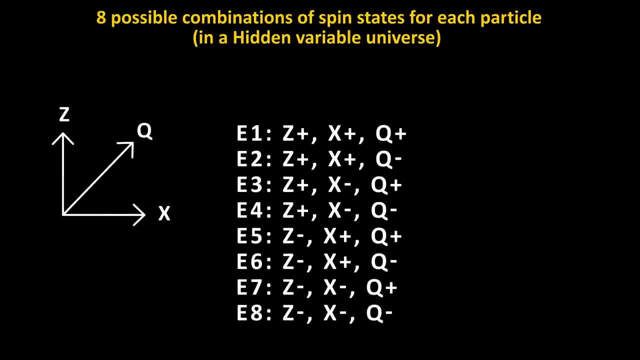 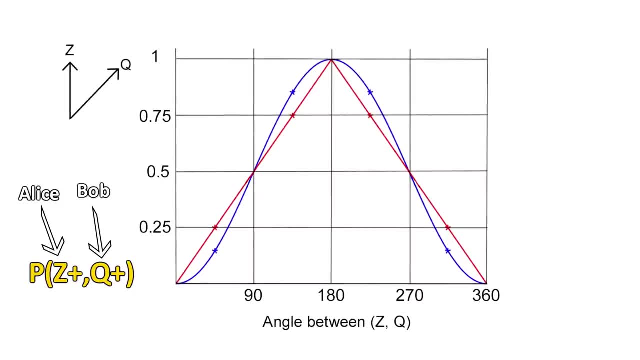 measurements as those change, changes are being made. Bell proved that quantum mechanics predicted stronger statistical correlations in the outcomes of these measurements than any hidden variable theory possibly could. I made a video about how Bell's inequality works if you want to learn more about this. 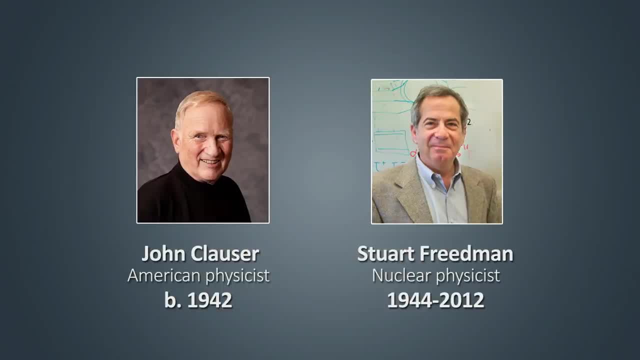 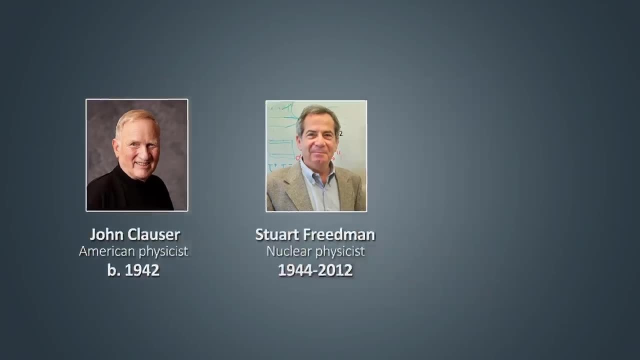 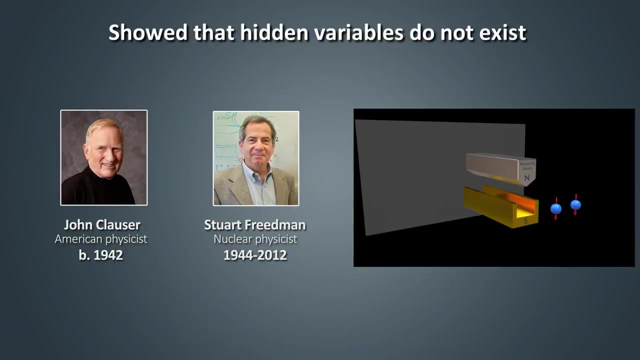 Suffice it to say that when Bell's experiment was first done in a lab in the 1970s by physicists John Clouser and Stuart Friedman at the University of California, Berkeley, it showed that there was no sign of hidden variables and that, indeed, outcomes are determined only by the act of 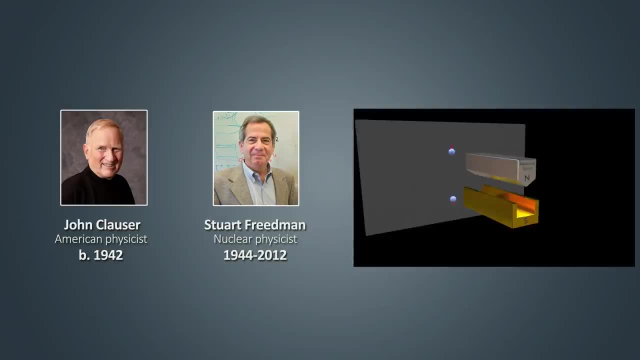 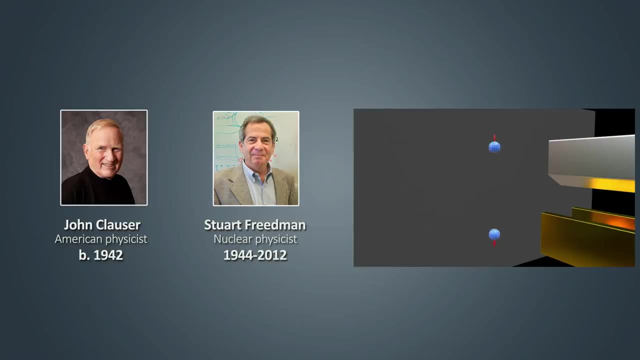 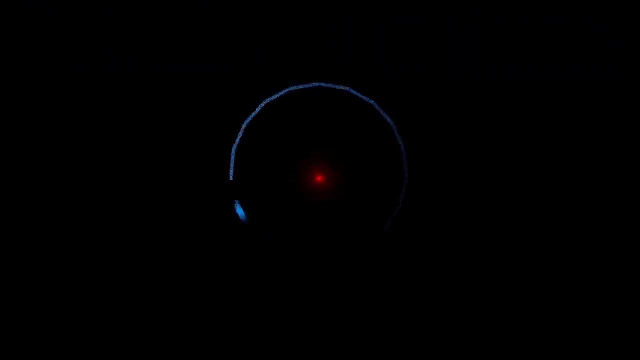 measurement itself, And in the ensuing years, this aspect of quantum mechanics has been proven to be correct over and over again. Bohr was right and EPR were wrong. Now you might be thinking: how exactly do you entangle two quantum objects? to begin with, The simplest way to make these is to 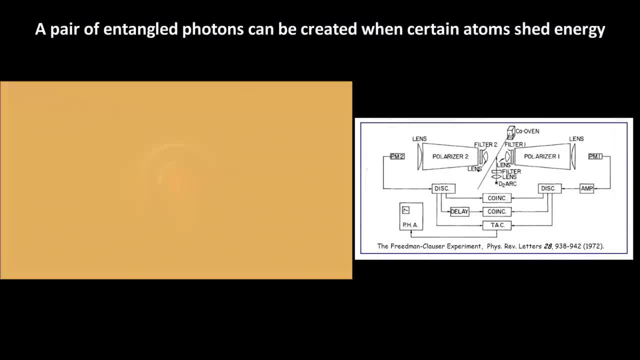 entangle them from birth Like twins, you could say. Typically you would entangle them from birth to birth. Typically, researchers make the pair of photons in a single quantum jump, For example, when an atom that has been given some extra energy sheds it by emitting two photons at once. There are clever. 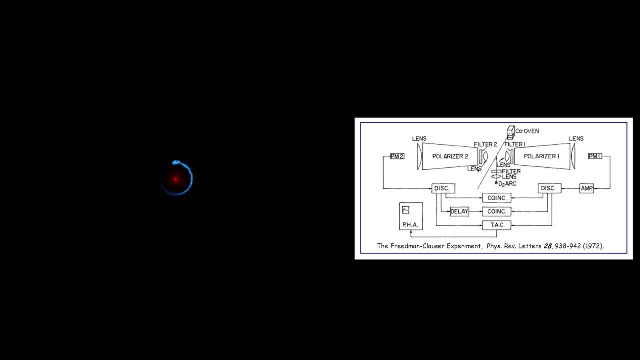 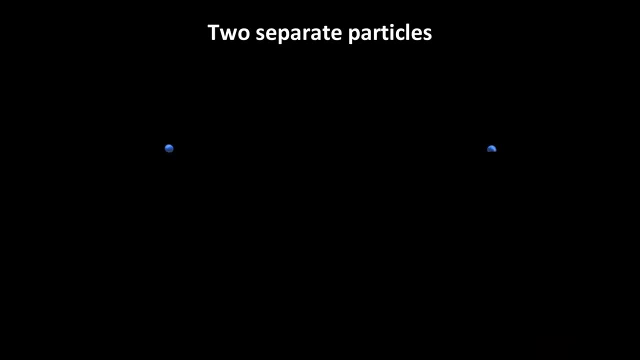 ways of doing this with lasers, which is how Friedman and Clouser did it, But there are other ways of creating entanglement between objects like atoms or electrons. The simplest way is to simply bring the particles together and let them interact. If you arrange for one particle to 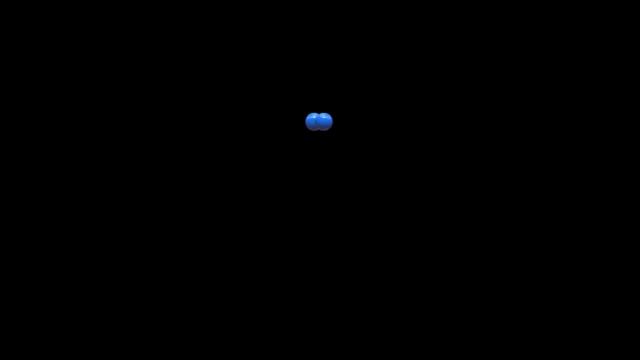 affect the final state of the second particle, then you can make the pair of photons in a single quantum jump. When you put the first particle in a quantum superposition, the pair of particles can end up in a joint superposition, An entangled pair. That's really what entanglement is: Quantum superposition of more than one object. 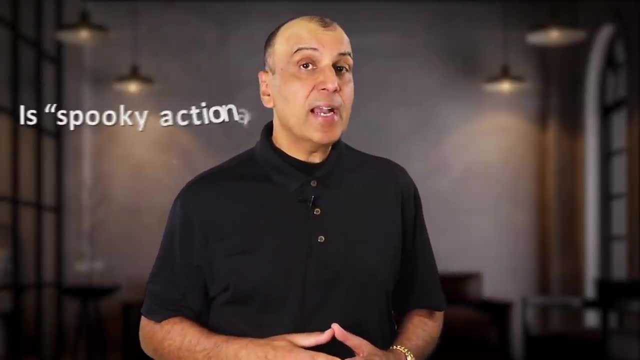 So do Bell tests mean that Einstein's spooky action at a distance is real? You might hear that claim, but it's not right. EPR were thinking about entanglement in the wrong way. That's not surprising, because what they were assuming was just common sense, So much so that the theory of the superposition is true. 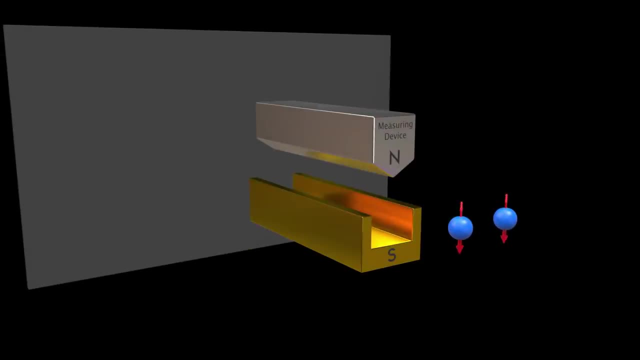 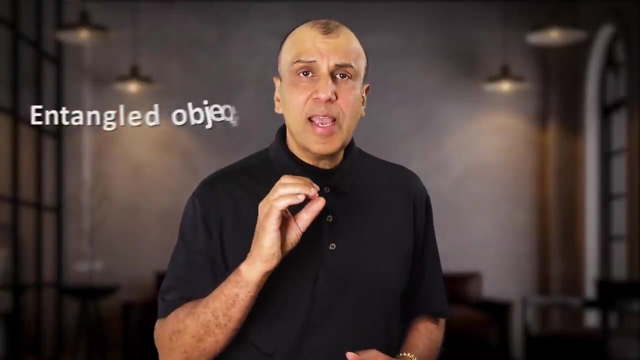 They were thinking of the two particles as separate objects. and why wouldn't they? After all, they are sent flying in opposite directions in space and in principle you can wait until they are many light years apart before measuring them. But once objects are entangled, they are not separate. They are in a sense two parts of a single object. Here's what that means. In quantum mechanics, objects are described by wave functions. These are mathematical expressions of the wave functions of two particles. 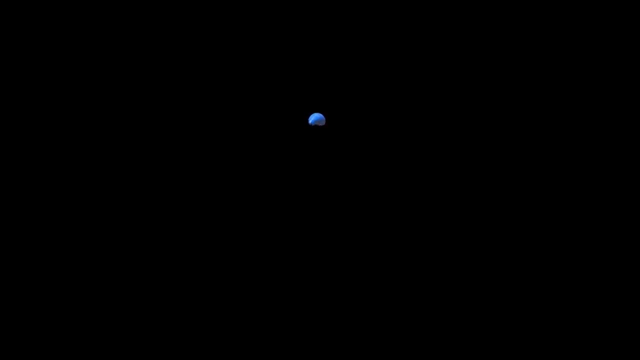 EPR is not a simple equation. It is more complex, While quantum mechanics is more complex than quantum mechanics. It is not a simple answer. It is a simple question. Some people are very similar, Others are very similar. expressions that encapsulate all that can be said about the object. 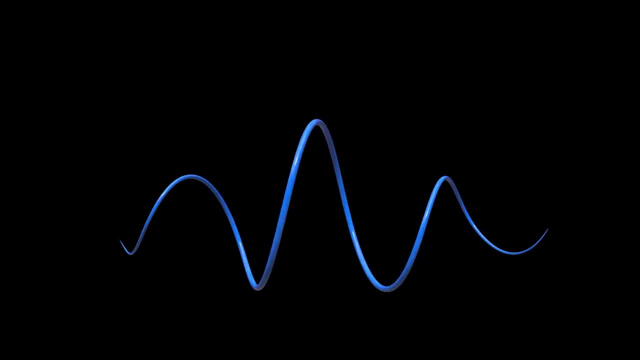 This wave function can be spread out in space. This is why particles can act as if they are waves. Yet if we entangle two particles, they are then described by a single wave function. And since two entangled objects are being described by the same wave function, they 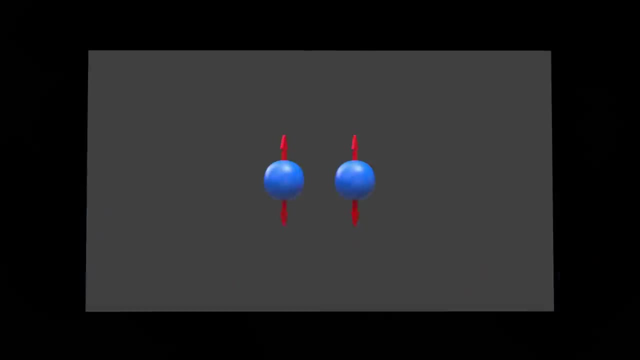 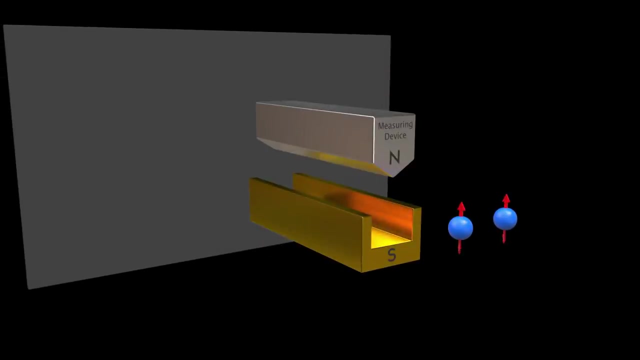 are, mathematically speaking, the same object. That's really what entanglement means, And it's why the particles' properties are then interdependent. If you do something to one of the particles, such as measure it, you change the wave function. 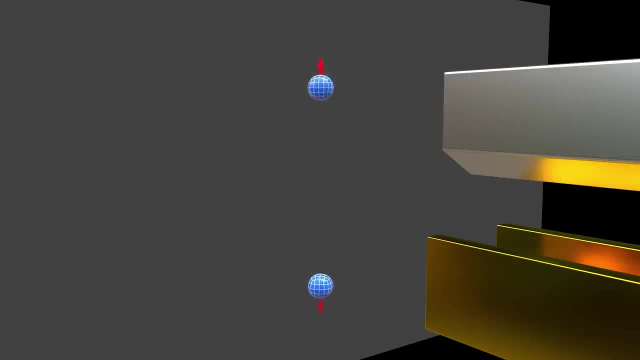 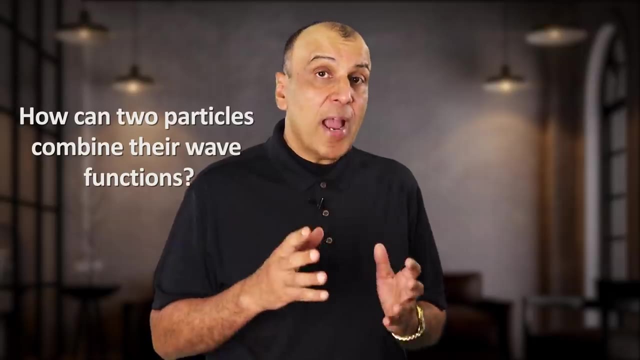 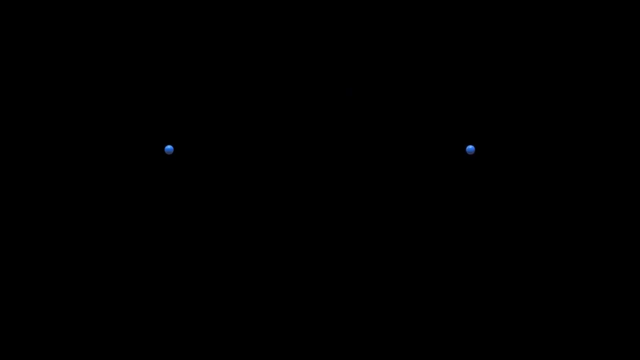 and so you alter the other particle too, since it is also described by the same wave function. Now the question you might ask is: how can two initially separate particles, by interacting, somehow combine their two wave functions into one? It really comes down to the math. 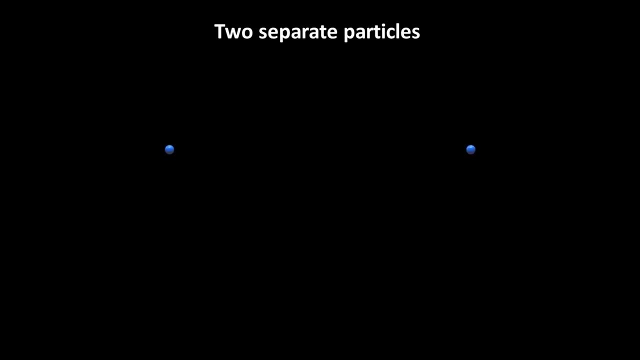 Before the particles interact we can separate the wave functions of the whole system of both particles into a part that describes particle 1 and a part that describes particle 2. But after they've interacted that's no longer true. We can't point to any part of the total wave function and say that bit is particle. 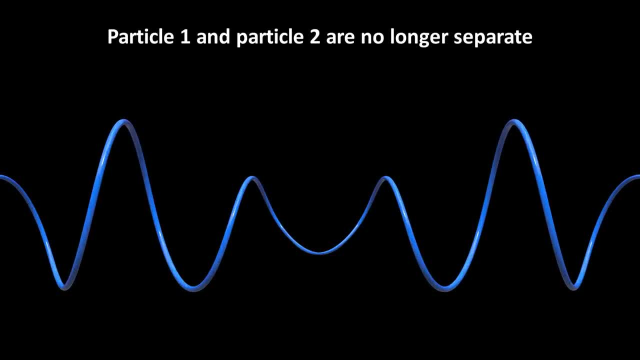 1, and the other bit is particle 2. This mixing up happens for almost any kind of interaction between them, So once two particles are entangled, we can't say anything about one of them without considering the whole wave function. It is as if they are interspersed. 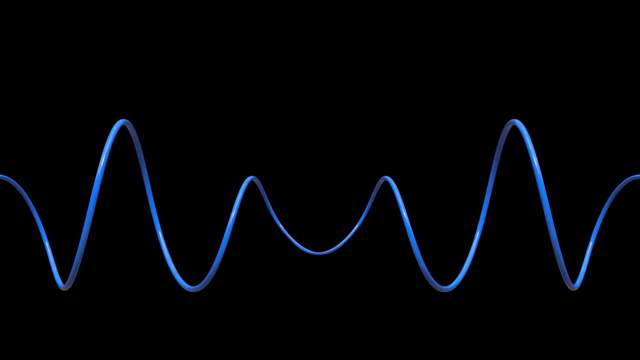 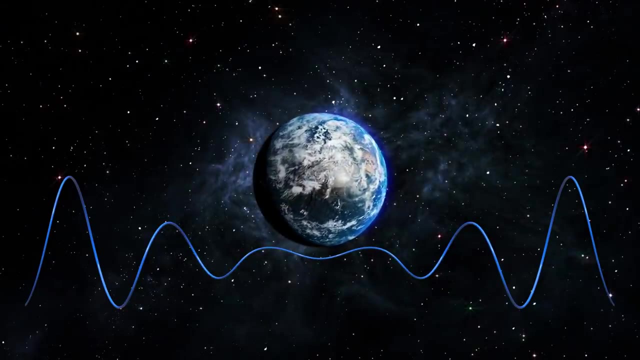 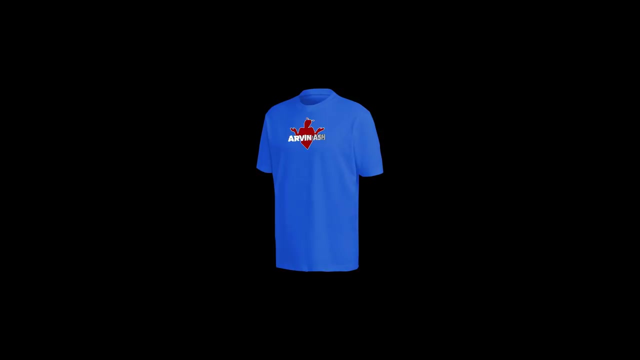 But their properties are now spread out over both. This is why it doesn't matter how far apart entangled particles are located. They're still interwoven by their joint wave function. That's the really strange thing. We are used to properties of an object being in or on that object. 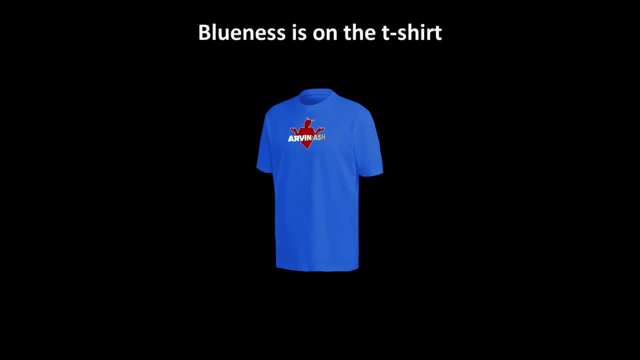 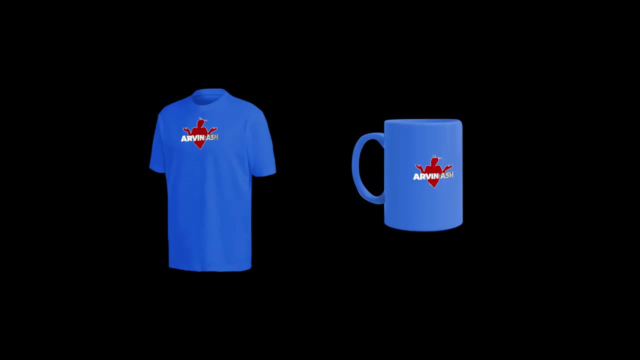 If my t-shirt is blue, the blueness is on the t-shirt, It's localized there. If I have a coffee mug, that's blue, that's the coffee mug's blueness, not the t-shirt's. But for entangled quantum objects, their properties can be non-local, spread between both objects. 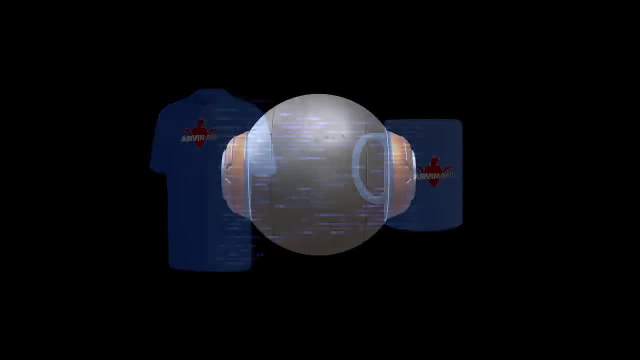 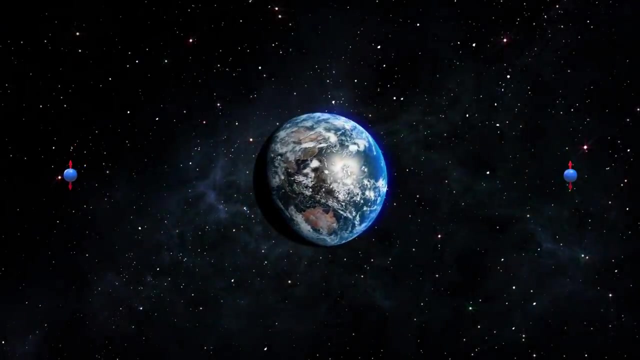 Some of the t-shirt's blueness can be in the coffee mugs, and vice versa. This brings us to why entanglement is at the heart of quantum mechanics, Because what it tells us is that the quantum world has a feature called non-locality. 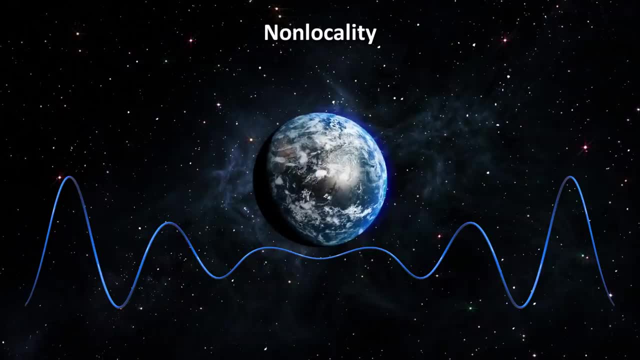 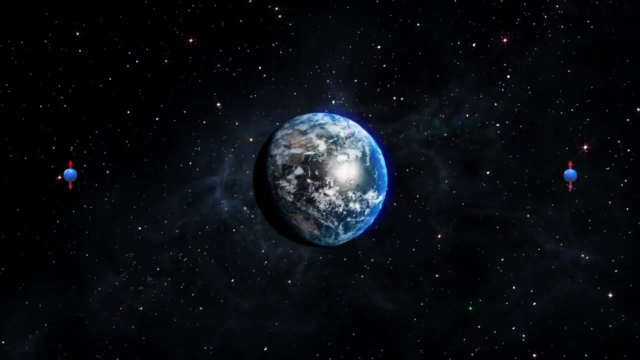 Things at one place don't depend just on what happens in the neighborhood of that place, as they do in the classical world. There seems to be a non-locality. There seems to be an instantaneous connection between different regions and particles, regardless of how far apart they are. 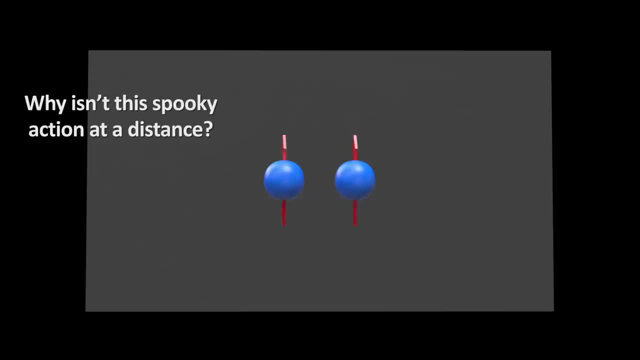 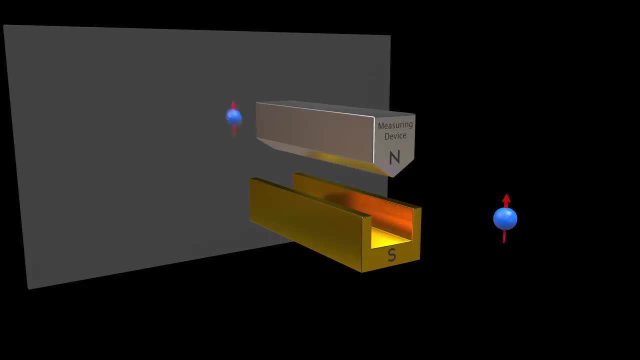 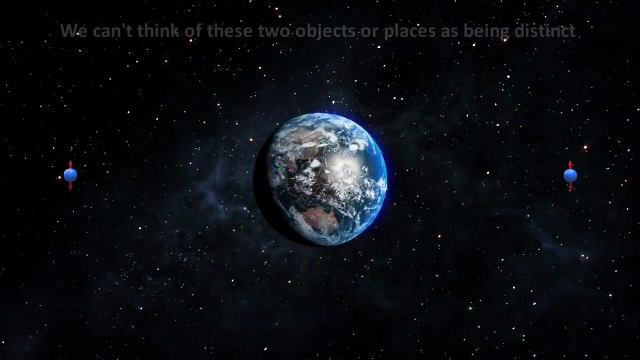 Why isn't this spooky action at a distance, then? That's because Einstein's picture was something at one place somehow transmitting its effects to another place faster than light. But quantum non-locality is an alternative to that picture. What it really says is that we can't think of those two places as being distinct. 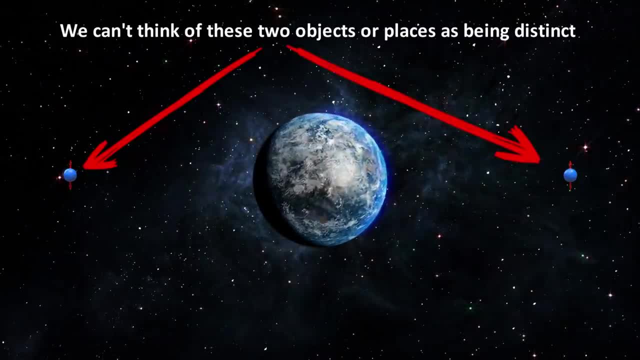 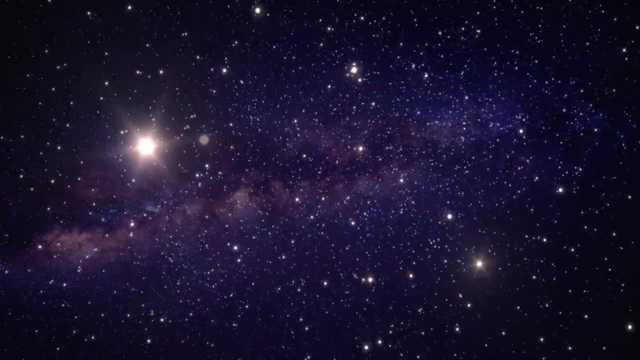 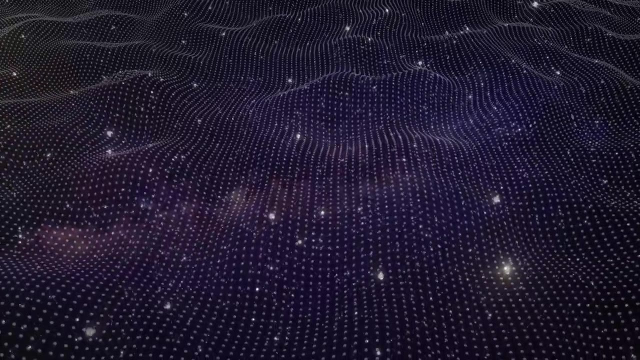 Quantum mechanics collapses them into a system. That's what it tells us. In this sense, quantum mechanics seems to make nonsense of our normal sense of space. In fact, some researchers suspect that quantum entanglement is more fundamental than space itself, And that our notion of space actually emerges from the quantum entanglements that connect. 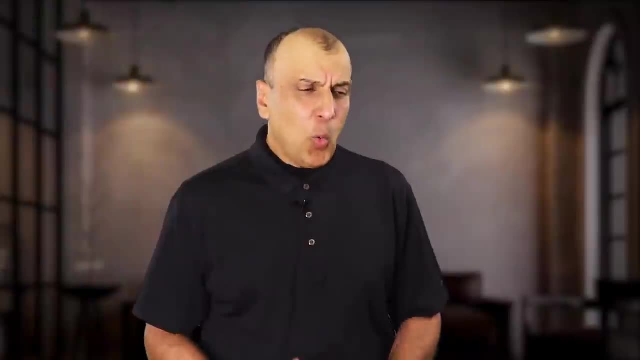 objects in a vast web of interaction. What about using quantum entanglement for communication? It's tempting to imagine that entanglement will let us communicate faster than light. Let's say we make a pair of entangled particles and separate them by thousands of miles. so 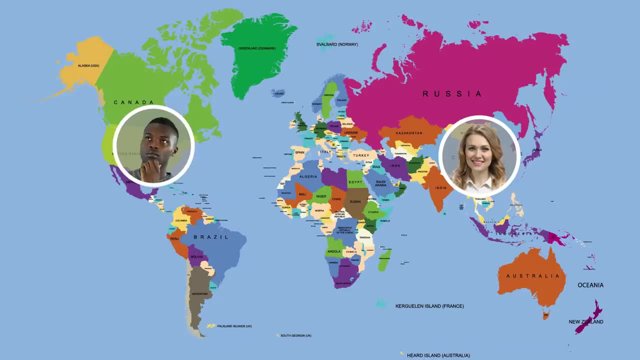 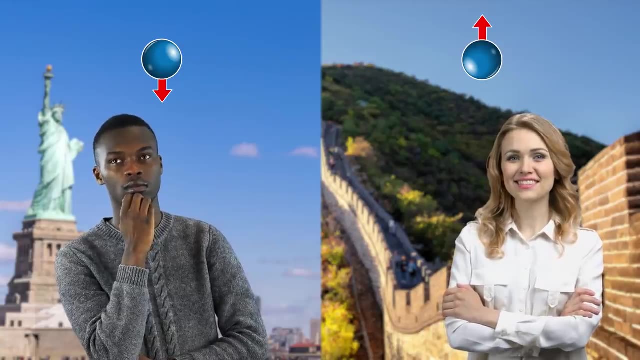 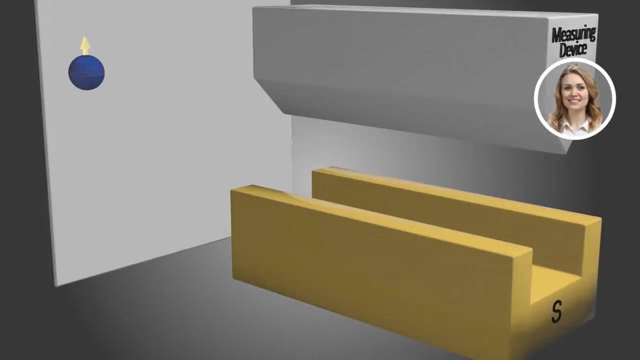 that Alice has particle 1 in China and Bob has particle 2 in the US. If Bob takes a measurement in the US, doesn't that mean Alice's particle in China is instantly affected? Well, yes, it seems so, But when Alice measures her particle it will seem like a random collapse to her. 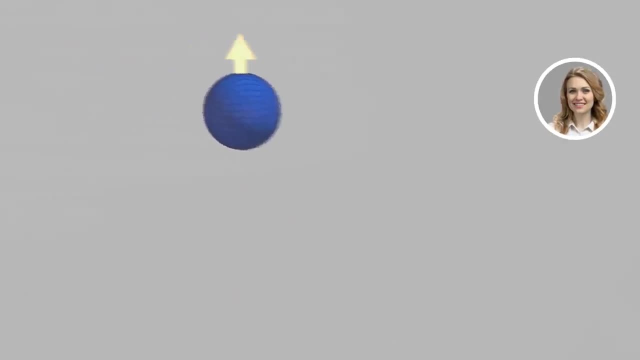 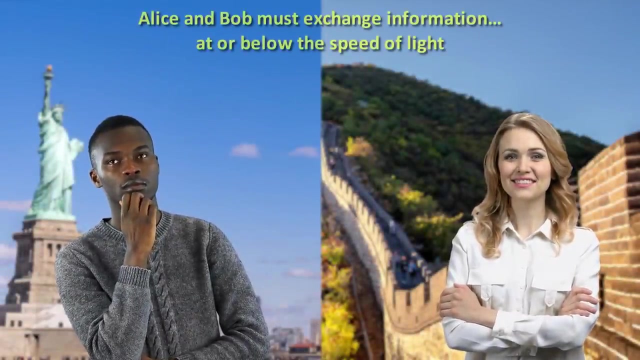 There's nothing meaningful about a measurement that Alice makes until she finds out how much it correlates with what Bob measured, And the only way to do that is by exchanging information about their measurements By sending an ordinary message, Email, snail mail, carrier: pigeon.